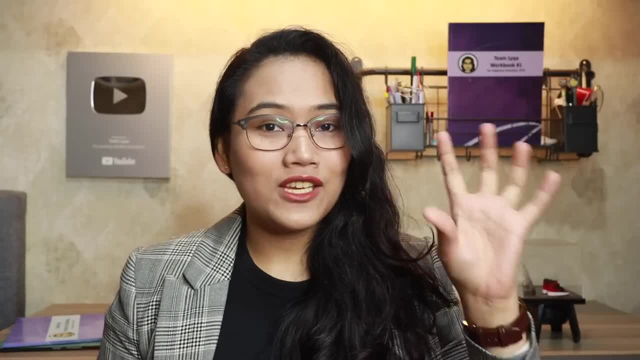 your exam is, And when you see the pie chart, you're excited because it's a bonus to you. And in order for me to explain this better, I'm going to switch over to my PC. I'll see you in a bit. 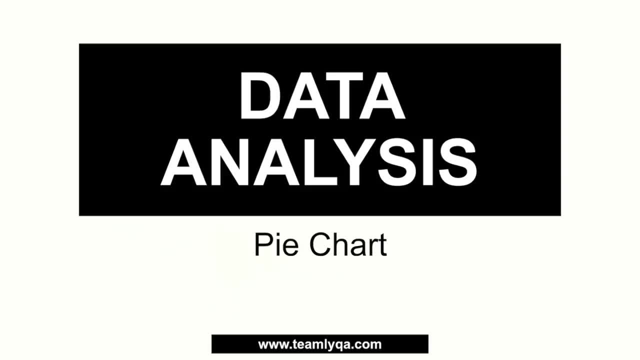 This is our lecture on data analysis, specifically on pie chart, And if you haven't seen my lecture on bar graphs, it's kind of like that- I'm going to give you a couple of- well, a bunch of questions with different difficulties, starting with the easy and then the average and then our hard. 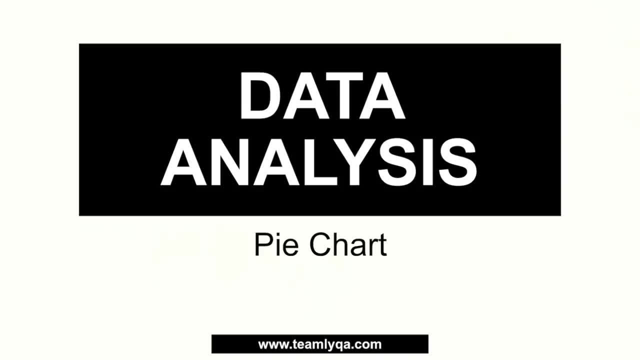 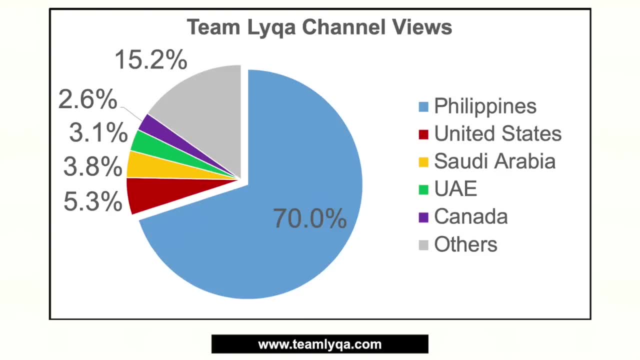 questions. So I'm trying to cover as many types of questions that you can expect, and I'll discuss then how I solve them in the exam. Okay, So this is what we call a pie chart. Basically, you have a big circle and then the entire pie, or the entire circle, has something that corresponds. 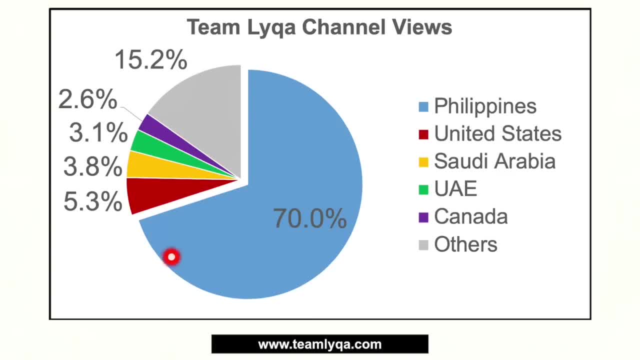 okay, Which is 100%. Basically, that's everything. The total is 100%. All of it would be the circle. Now, what are the parts? These parts are the share. The share of a thing, a category or anything like that goes to that 100%. So, for example, this title of our chart, which is very 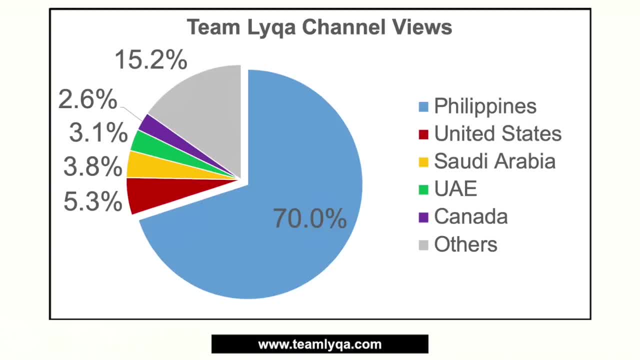 important. it says here: team like a channel view. So this is just a mock-up, like a sample for you. If it says team like a channel views, it means all of that would be the total number of views of the channel for that given period. right Now, every part, we're here in our legend table. 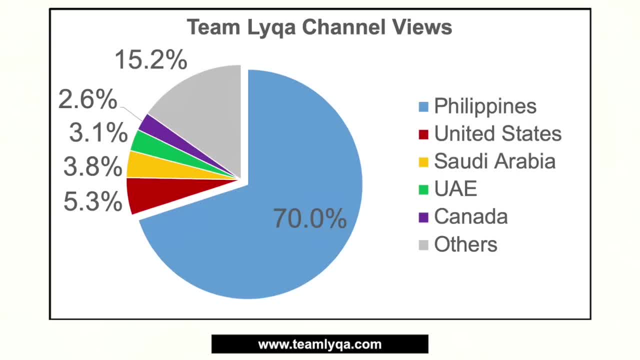 they have different colors, sometimes different markings or shades. It says here what countries? So this is the 70%. It means that 70% of the total of all the viewers in the team- like a channel- it's no longer far from reality- comes from the Philippines. This 5.3% is from the United States. 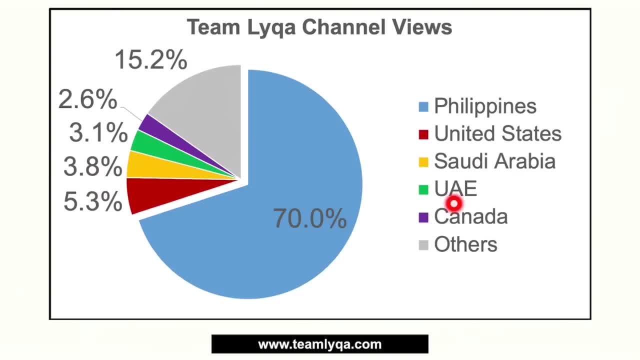 3.8% from Saudi Arabia, 3.1% from the UAE, 2.6% from Canada and 15.2% is others. If it says others, it means every other country out there that has views from that country. Okay, So it's. 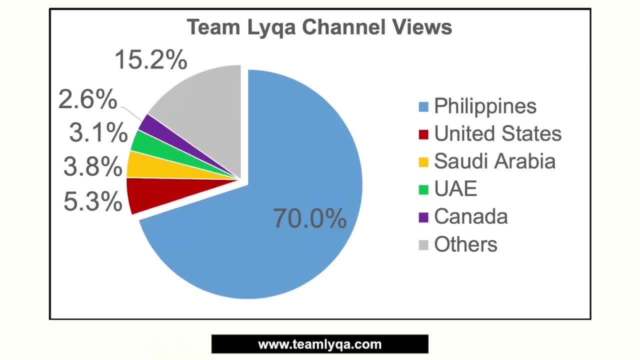 kind of like. this is really the situation in the Philippines sa Team Laika channel, pag off-season ang review, So yun walang paparating ng mga exam. So medyo doon ko kinuha itong statistics na ito. 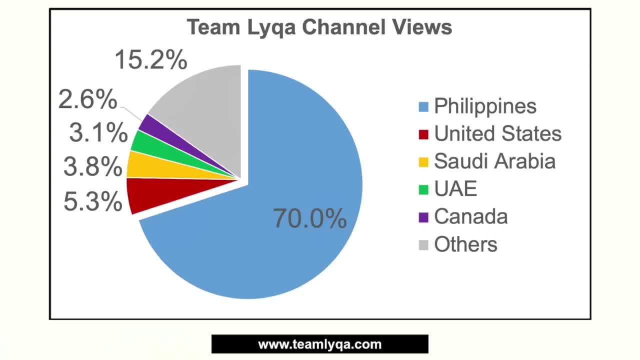 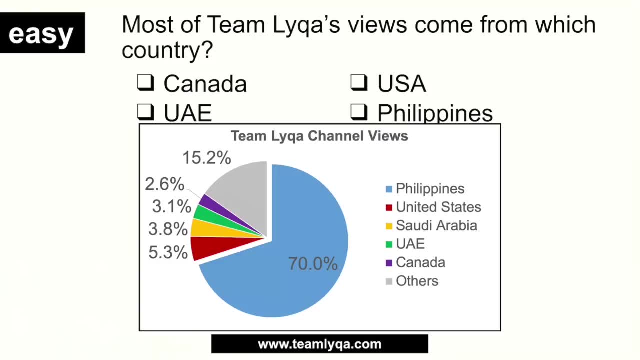 Okay, Now out of this chart right here, may mga posibleng questions na lumabas. Okay, Ang pinaka-common na question would be something like this: Sabi sa easy round natin, most of Team Laika's views come from which country? 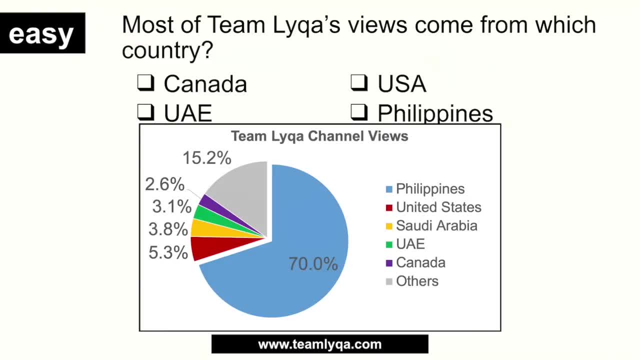 So sabi most or mas marami, karamihan sa views daw ng Team Laika come from which country? Now, ang pinaka-daling way for you to see that is through the chart. ano yung may pinaka-malaking slice? 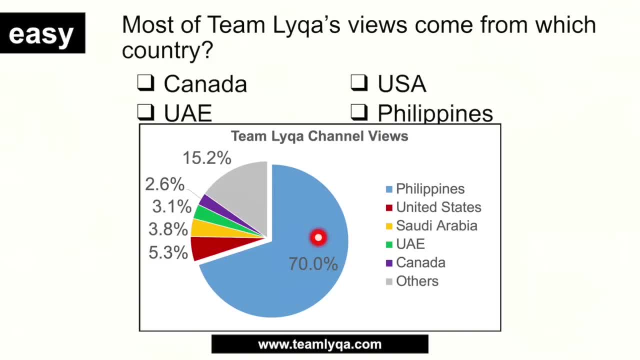 Okay. So even if you don't look at the values, you would see right away: higit sa kalahati pa nga 70% is from the Philippines. So the answer here would be yung Philippines Sen yung country with the most views. 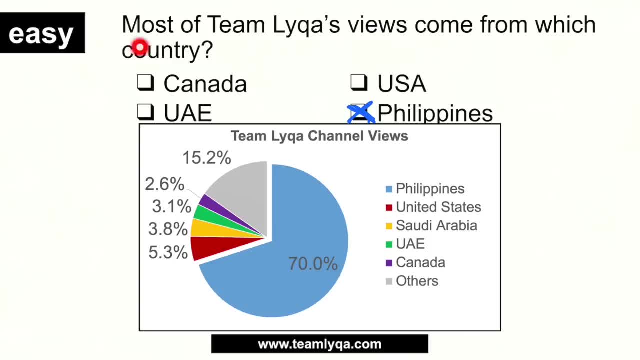 Okay, Minsan tinatanong yung least, Minsan tinatanong yung pinaka-konte, Minsan tinatanong yung pinaka-marami, Minsan tinatanong yung second. 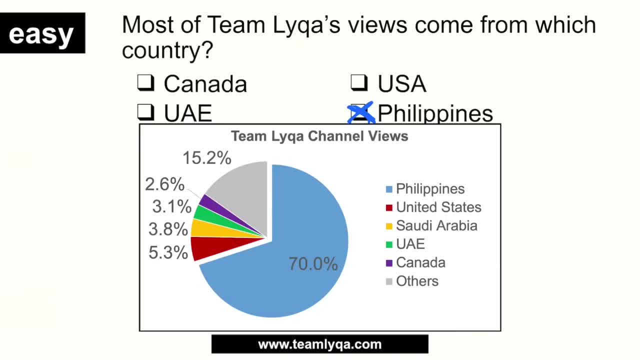 Second least or second most, All of those things. ganito yung titinan nyo lang, titinan nyo yung number niya, ano yung ranking niya, At dahil most ang hinahanap 70, yung pinaka-marami. 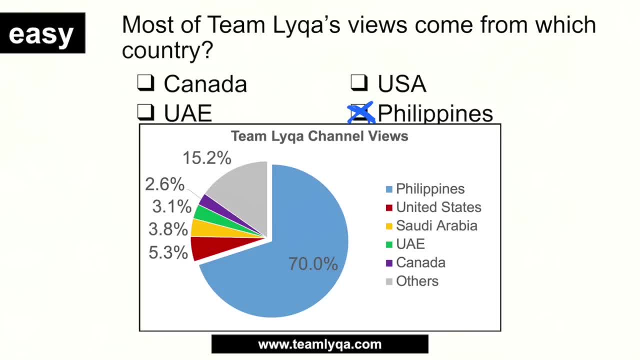 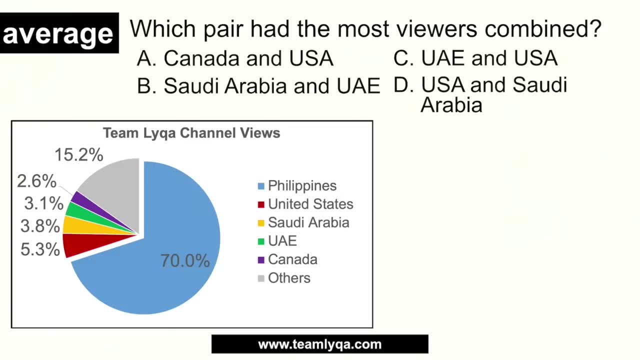 Philippines ang sagot. So basically pinagbabangga-bangga mo lang yung mga data. Ito yung type ng easy question. Now things change kapag ganito na Average. So sabi sa tanong: 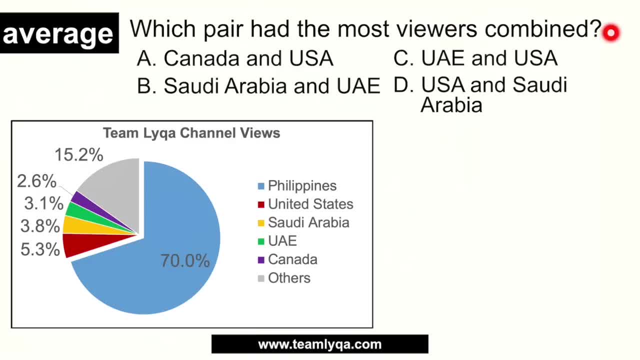 which pair has the most viewers combined? Okay, So dahil combined yan ibig sabihin pagsasamahin mo yung pair ng mga countries na ito, So it will require you a little bit of ano ba mass na rin. 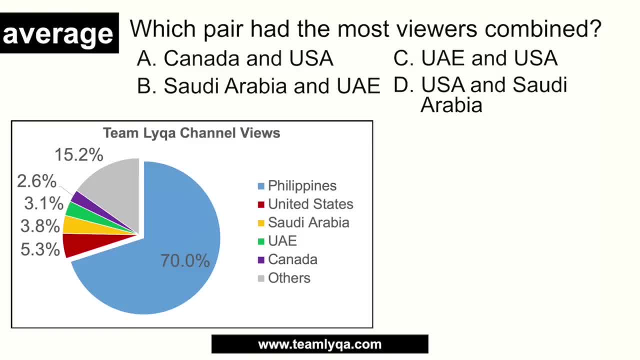 So simulan natin sa Canada and USA. Ang Canada is yung purple natin, which is 2.6.. Tapos, idadagdag natin, kasi combined is addition no 2.6, idadagdag natin yung sa USA, which is yung color red, 5.3. 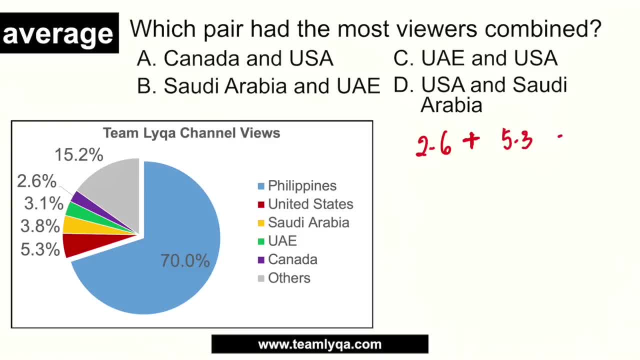 Okay, Yan, yung first one. So this will be 7.. So this will be 7.9.. Okay, Now you don't need to write this down. The more that you do this, the faster you'll get no. 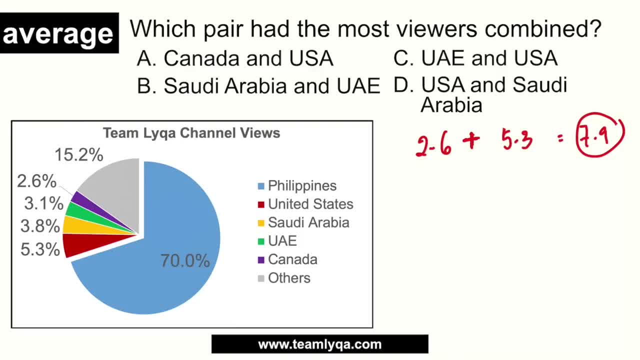 Pag minsan patingin-tingin ka na lang sa exam. Pero kung nasisimula pa lang kayo, it will do you well to write it. Next yung Saudi Arabia and UAE. natin Saudi Arabia is yellow. 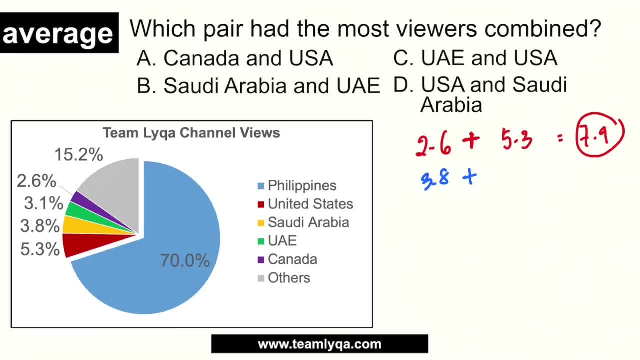 That is 3.8.. Tapos idadagdag natin yung UAE. UAE is green, That is 3.1.. Again, i-add lang natin 6.9.. So hindi na siya pwede. 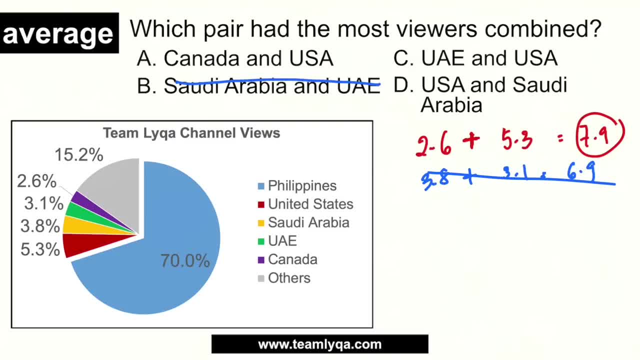 Talo na siya, Kasi 7.9 yung isa, So hindi na ito pwedeng sagot. That's how I cancel answers sa exam. Next we have yung UAE and USA. Ang UAE natin is 3.1.. 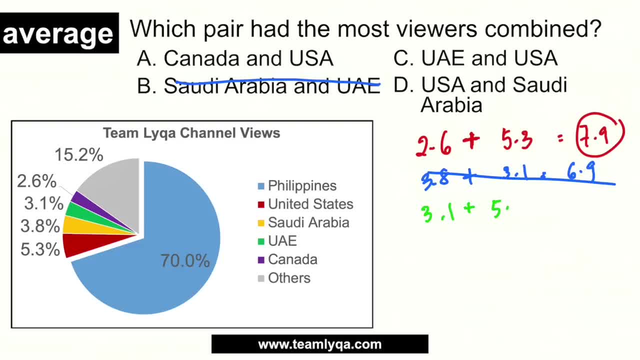 Ang USA is 5.3. So i-add natin sila. This will be 8.4.. So tanggal na rin yung letter A, Hindi na siya pwede. Ang candidate na natin is letter C. 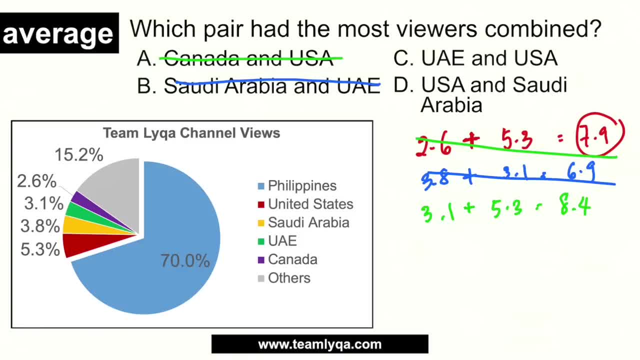 Letter D na lang. Just to make sure, Letter D. We have USA, which is again 5.3. And yung ating Saudi Arabia, Saudi Arabia, is 3.8.. So pag-i-add na naman natin siya. 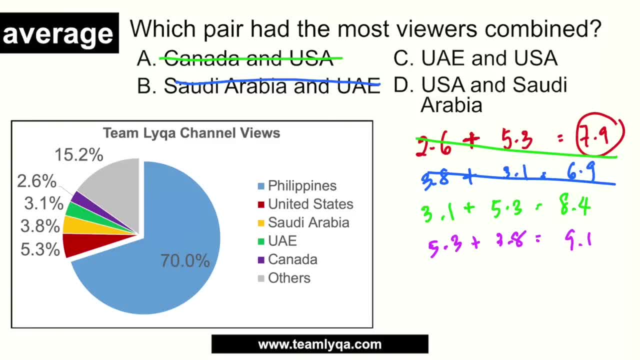 So we have 9.1.. Now the way that I do this is I first combine yung buong number, So 5 plus D is 8.. And then yung 0.3 plus 0.8, that is 1.1.. 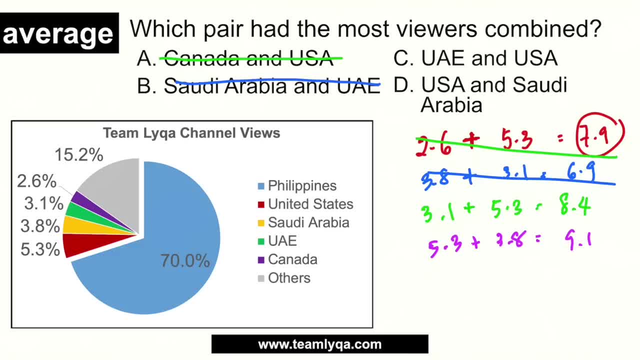 I-add ko lang siya doon. So 9.1 ang sagot. So if you notice yung 9.1 ay mas malakay siya kaysa sa 8.4.. So ibig sabihin hindi ito ang tamang sagot. 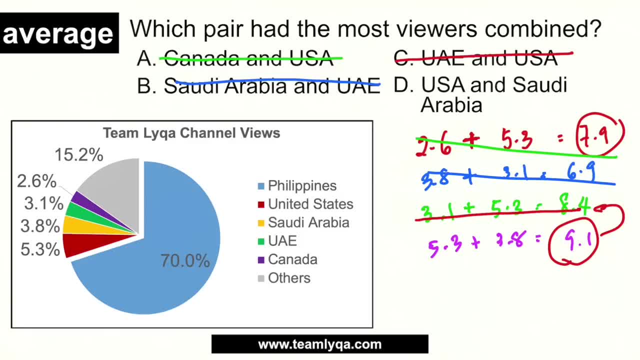 Ang tamang sagot natin is letter D: USA and Saudi Arabia. Sila yung may pinakamarami na viewers combined. Okay, So again, may unti ng operations required. It will require you to add a few things. 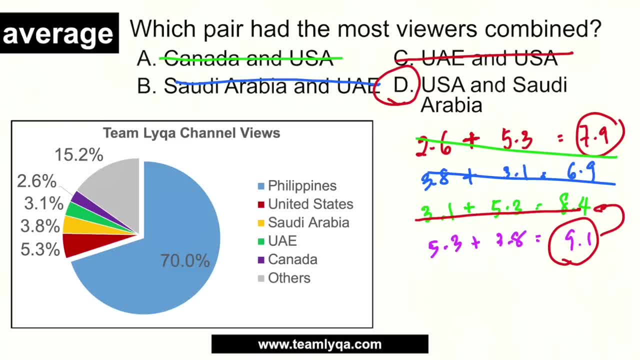 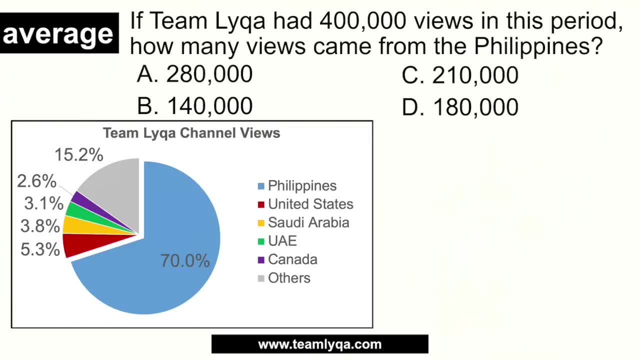 Yan, yung mga klase ng mga average or moderate level na difficulty, na questions. Okay, Let's try another type. no, Sabi ito. if Team Laika had 400,000 views in this period, how many views came from the Philippines? 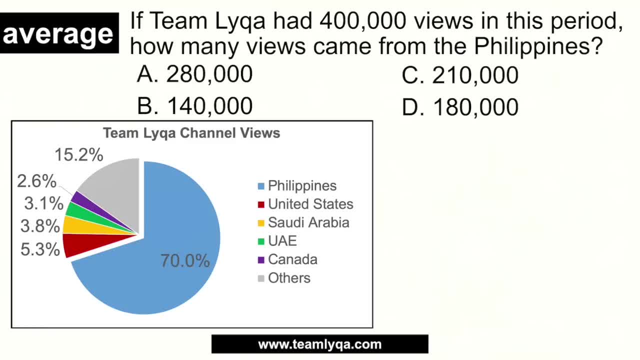 Okay, Ito again you will have to do a little bit of math. Sabi dito sa Tagalog: kung 400,000 daw ang total na views, ilan ang views na galing sa Pilipinas. 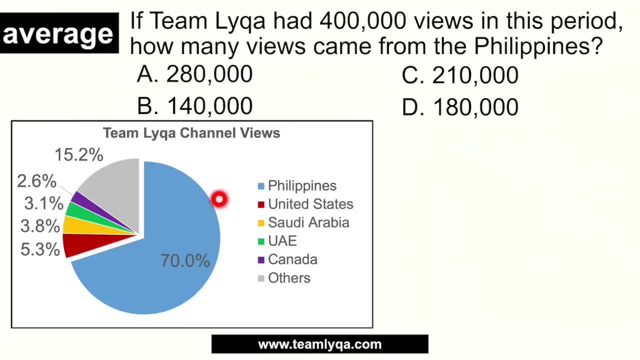 So anong ibig sabihin yan? Ibig sabihin yan: yung buong pie right here. ang total ng buong pie na yan is 400,000.. Okay, 400K yan, Pero ang kinukuha lang natin ngayon would be this part right here, yung 70%. 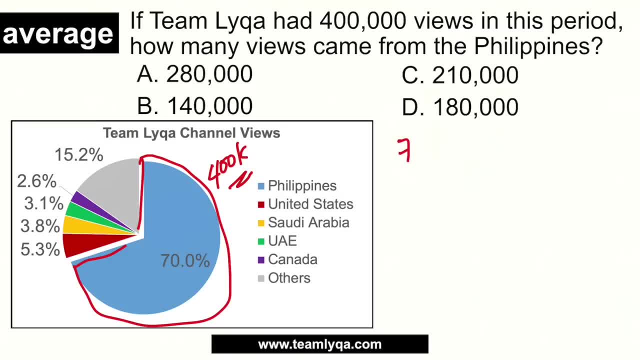 So ang gagawin natin dito is basically yung tanong: what is 70% of 400,000?? Okay, Now again you can do it, na ganyan, I-multiply natin siya. 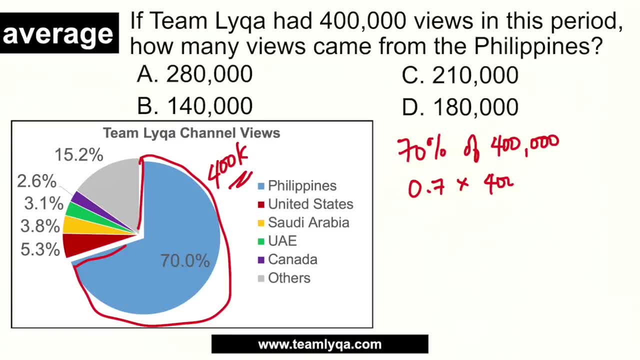 So 0.7 times 400,000.. You can do it like that: I-multiply mo lang siya, Or what I do sa percentage questions, and if you haven't seen my video on my shortcut, lalo na kung walang calculator na ginagamit sa exam. 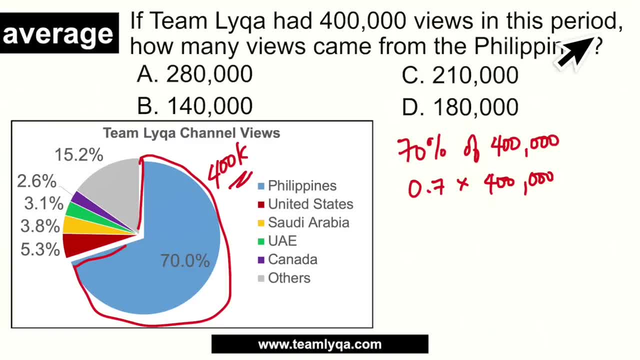 panoorin nyo na lang sa taas. I-link ko na lang dun sa upper right corner, dun sa i-button there. no, Pero ang ginagawa ko kasi dyan, kung ako magkocompute, lalo na walang calculator, yung exam, iniisip po lang muna. ano, ang 70% ng 100,000 muna. 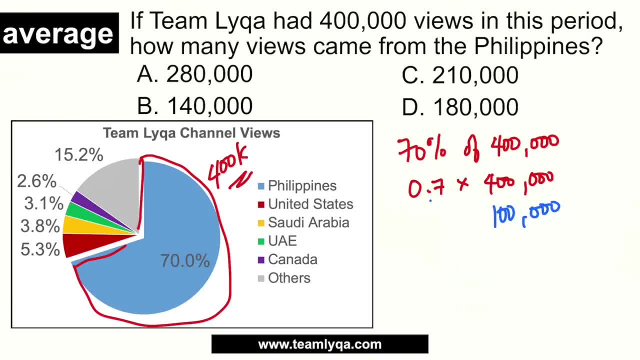 Now ang 100,000, okay, ang 70% niyan, very easy naman, It's 70,000.. Kasi ang 70% ng 100 ay 70.. So dalagdagan ko lang nung tatlong zero. 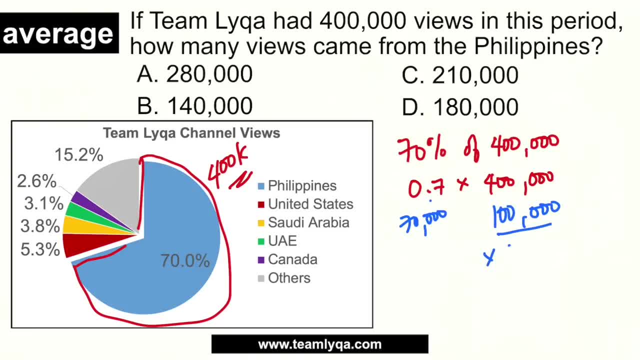 At dahil yung 100,000 ay apat, okay, apat niyan ang 400,000, ito times 4, ko lang din ito. This is something I can do mentally. So 70,000 times 4, that would give me 28,, 7,, 14,, 21,, 28.. 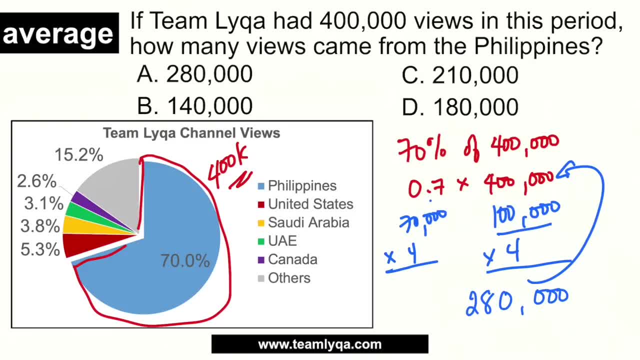 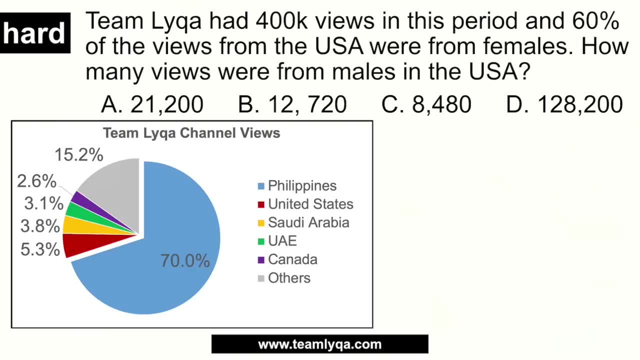 Tapos zero and three more zeros right there, So my answer is 280,000.. The answer is letter A. Okay, Now dito tayo sa hard question. natin. Sabi dito: Team Laika had 400,000 views in this period and 60% of the views from the USA were from females. 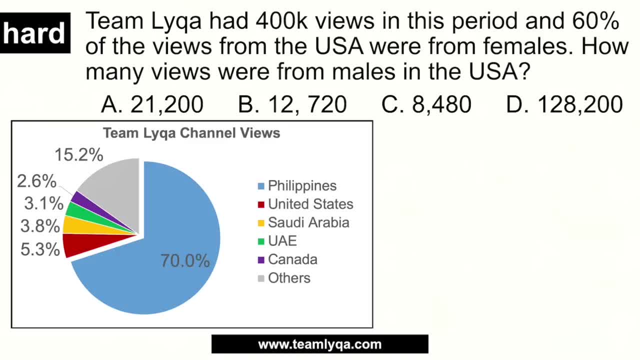 How many views were from males in the USA. Okay, So ito may step further siya, kasi hindi na lang yung share ng USA ang hinahanap. Ang hinahanap is how many were from males in the USA. Now, kung makikita ninyo, meron kang information dito, which is yung 400,000 total. 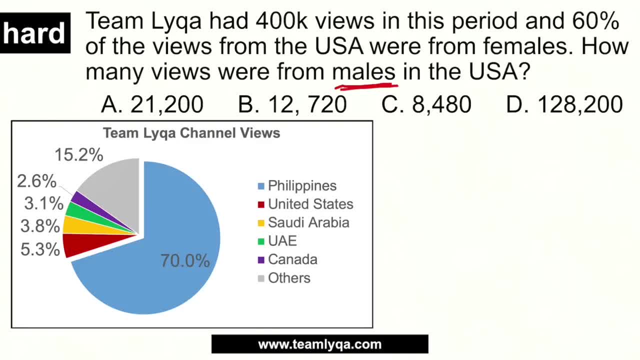 Okay, 400,000 total views and then 60% yung sa females. So ang tanong na here would be: ilan muna yung share ng USA. Now ang share ng USA would be 5.3%. 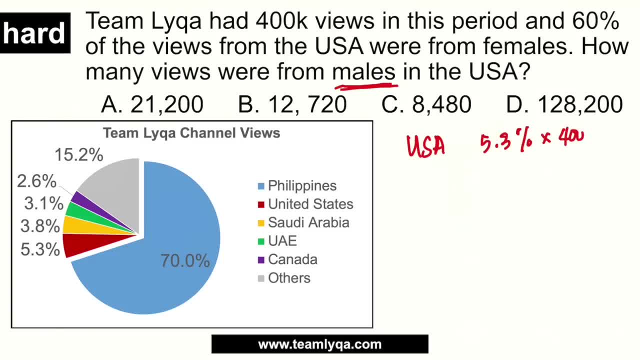 So 5.3% muna of 400,000.. Okay, Now ilan muna yung 5.3% ng 100,000? That would be 5,300.. Okay, Ito yung 5.3% ng 100,000.. 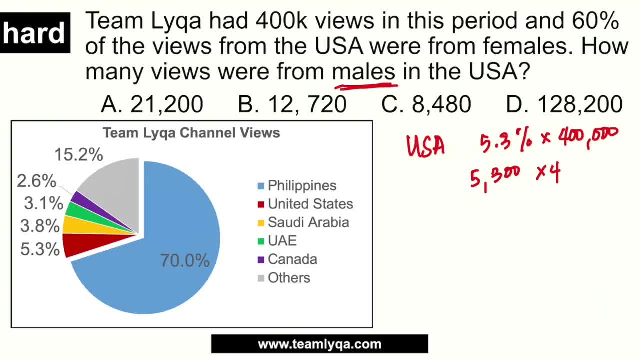 Ita times 4 ko lang din siya. Parang ginawa ko kanina, This is my style, no, But again you can do this. I-multiply nyo na lang. Pwede nyo rin gawin yun. 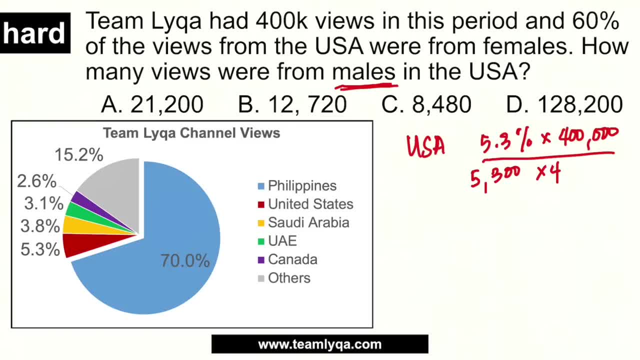 Sa akin lang Basta dali to mentally So ang ginagawa ko dito: apat na 5,000.. That would be 20,000.. Tapos apat din na 300. That would be 1,200.. 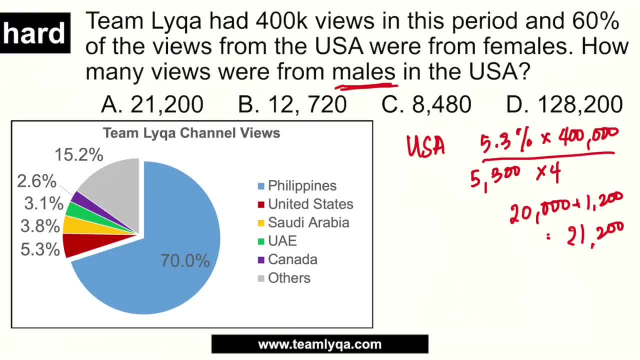 So my answer would be 21,200.. Yung total ng Hindi pa ito tapos ha. Ito ay number ng taong nanonood sa USA, Pero hindi pa tayo matatapos d'yon. Kasi ang hinahanap, ilan nyo daw yung lalaki. 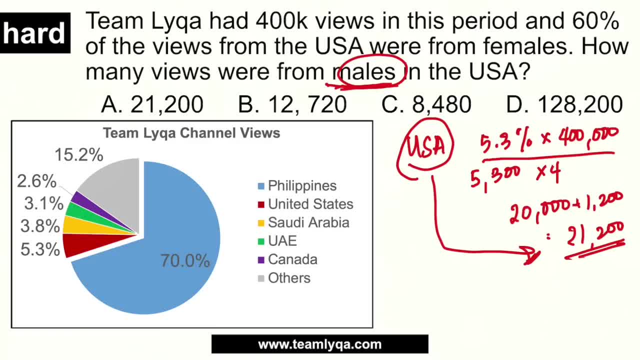 Now you can do two things. Number one: pwede nyo kuling yung 60% nito at ibawas ninyo sa 21,200.. Okay, Anong ibig sabihin ko doon? Again, what you're going to do here would be: 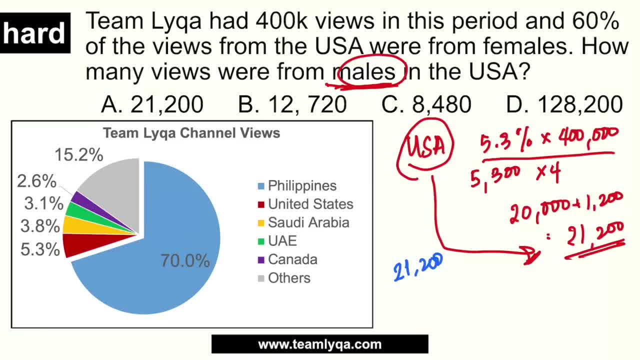 Ito yung option number one: 21,200.. Tapos times 0.6.. Tapos, kung ano man yung sagot mo dito, ima-minus mo d'yan. Okay, So 21,200 minus whatever that is. 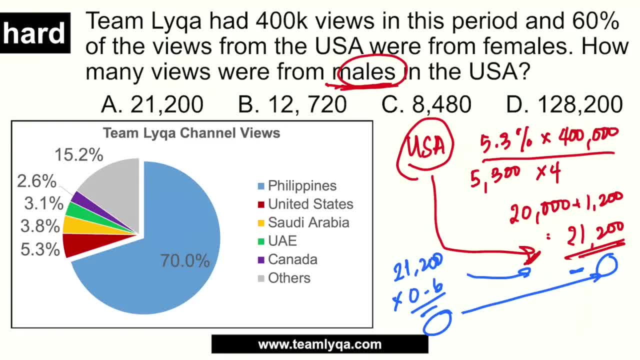 Okay, You can do it like that Or ang ginagawa ko na lang, kasi kung 0.6 or 60% yung babae, ang lalaki nyan would be yung 100% minus 60%. 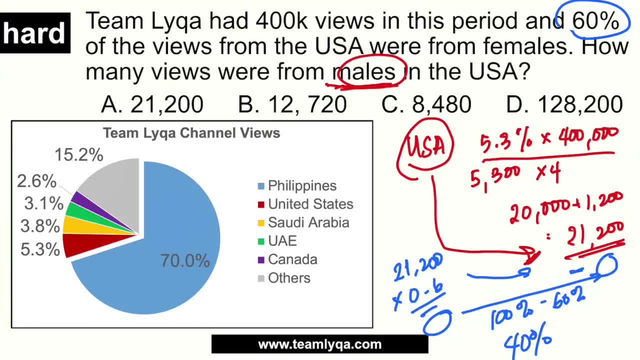 Kasi the rest would be 40%. Yan yung lalaki. So yung hinahanap mo ngayon would be 40% ng 21,200.. I just prefer this kasi mas unti na yung isosolve ko. 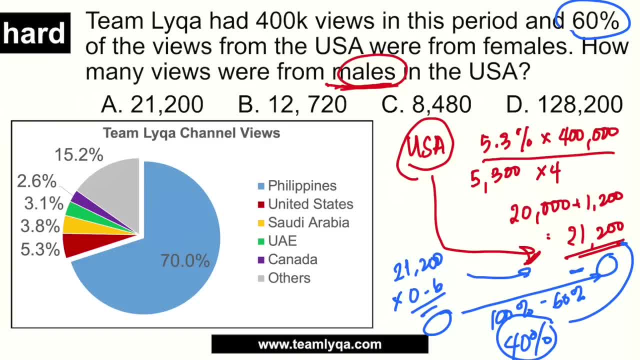 Imbis na i-multiply ko, kasi ma-minus ko pa i-didiretso ko na lang ng multiply sa 40%. Now again, ang gagawin ko na lang is: I will multiply this by 40%. Now, paano ko yun makukuha? 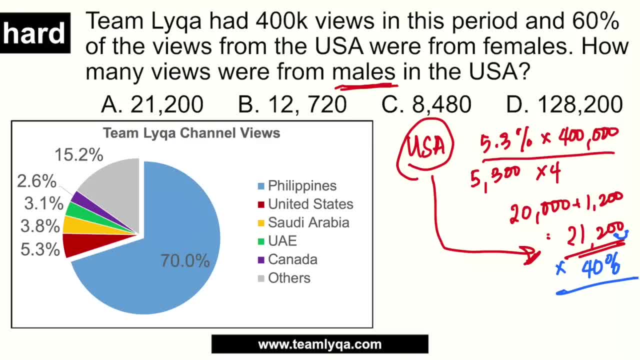 10%, muna Ang 10%. i-gagalaw ko lang yung decimal place sa isang beses, That is 2,120.. Basically ito ay i-multiply ko lang sa apat, So apat nito. 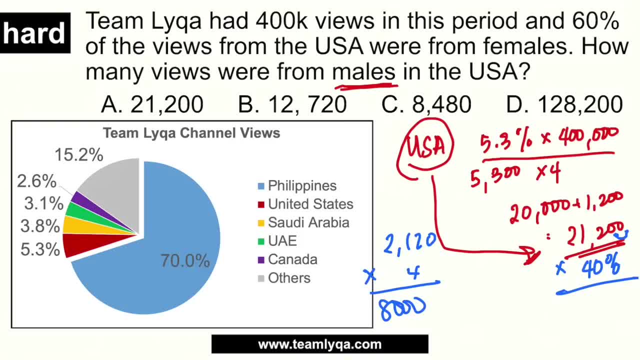 Okay, That would give me 8,000 right away. Tapos, Tapos plus apat na 120.. So 400 plus apat na 20,, 480.. So my answer now would be letter C 8,480.. 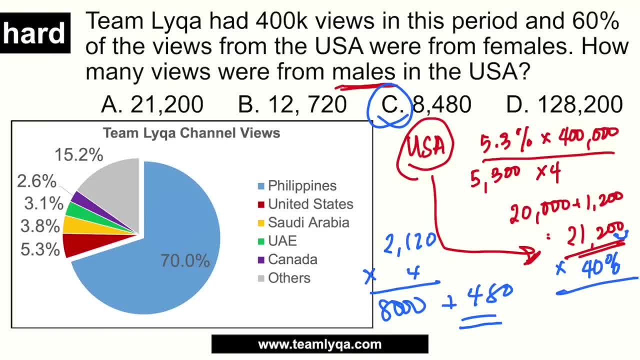 Okay, But again, kung gusto nyo, i-multiply like this, okay lang din. Pareho naman yung lalabas na sagot. This is just my way of doing it, kasi it's faster, Lalo na if you cannot use a calculator sa inyong exam. 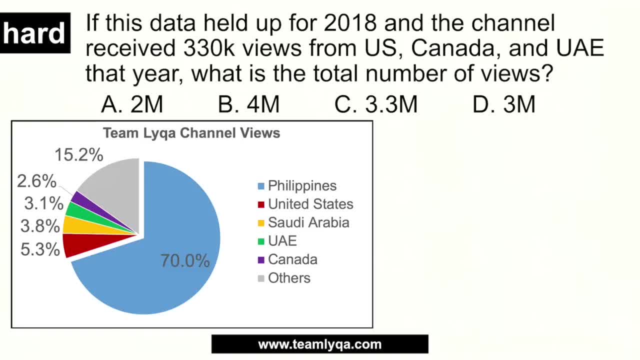 Okay, Now ito na yung last question natin dito. sa video na ito Sabi: if this data held up for 20 years or 2018, ibig sabihin ganito pa rin ang ratio sa buong 2018,. 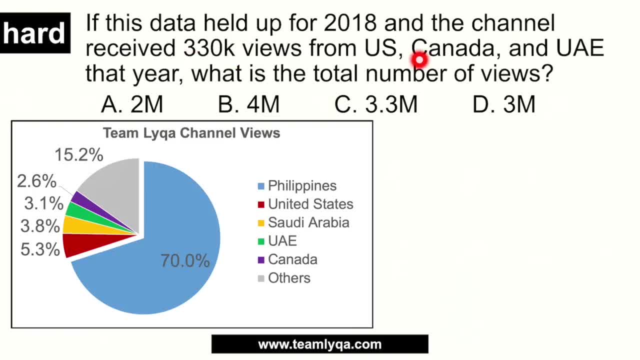 and the channel received 330,000 views from US, Canada and UAE that year. what is the total number of views? Okay, So ang sinasabi dito is yung views daw for 2018 ng US. ang US is 5.3,. 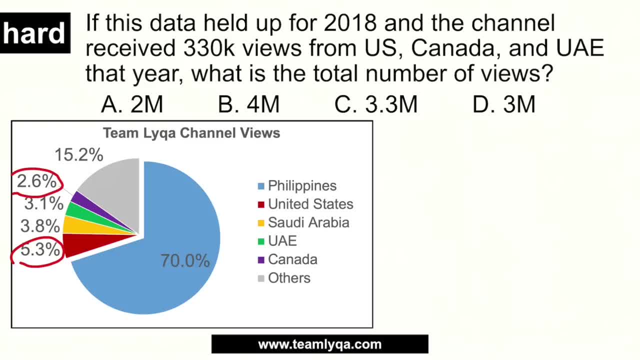 Canada- Canada natin is 2.6, and yung UAE ang UAE natin is 3.1.. So pag pinagsama-sama mo daw ito, ang total na views niya ay 330,000 views. 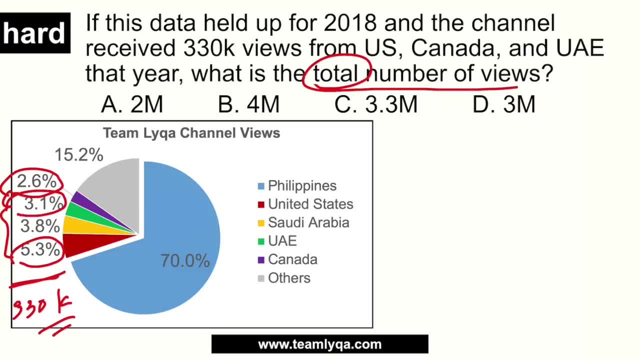 Okay, Ang hinahanap is the total number of views, Ibig sabihin yung buong 100%. Now, how do I get that? Ang pwede nyo maisip dito would be: ano muna ang percentage ng 330,000?. 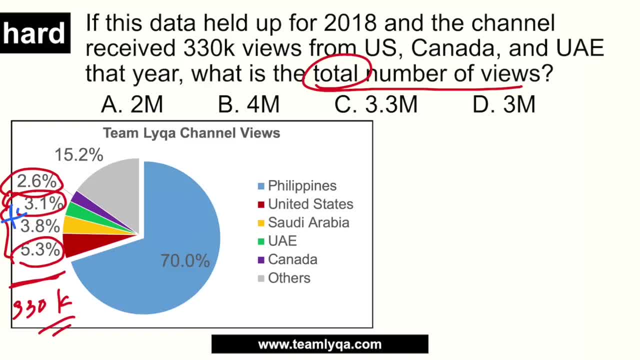 Ang percentage niyan. kung pagsasama-samahin ko itong tatlo na ito- 2.6 plus 3.1 plus 5.3, that would give me 11%. Okay, Paano ko yung nakuha? 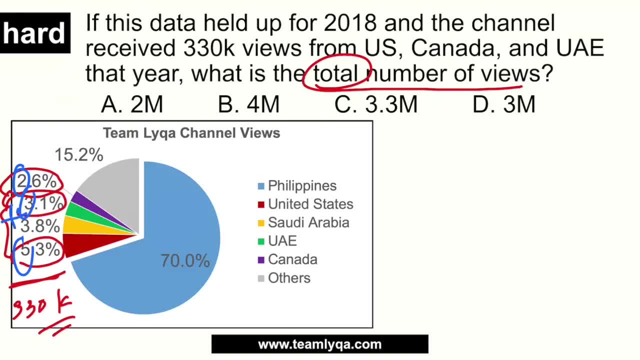 Basically pinagsama-sama ko muna yung whole number, So 2,, 3,, 5, that will give me 10.. And then pagsasama-samahin ko yung decimal 0.6, 0.1, eto, 10 na agad. yan, So 1.. 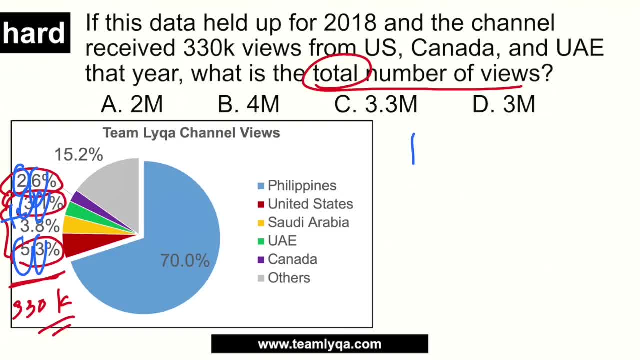 So yung 10, nalagyan ko ng isa pa 11%, So ibig sabihin 11% ang 330,000.. So ang tinatanong na lang is: if 11% ay 330,000,, ano yung kabuuan? What is 100% Okay? 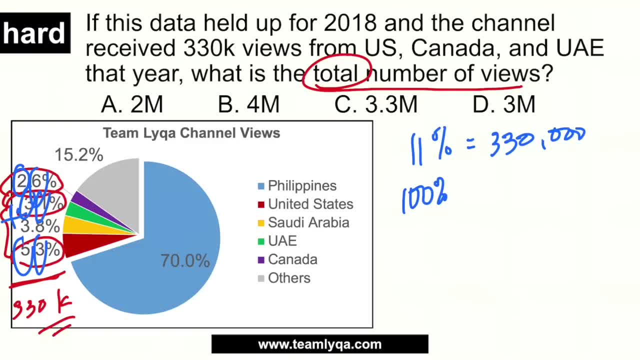 Now you can do it a couple of ways. Pwede mo sabihin na if 330,000 is 11%, of what number? what is that number? Okay, So pwede mo siyang gabing equation which would look like this: 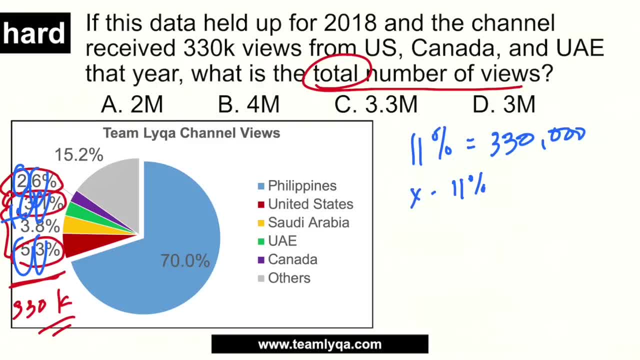 x times 11% is equal to 330,000.. Pwede nyo isolve like that. You just need a little bit of algebra. no, Pero ako kasi, and I teach this din in my video. I also did a revamp on this. 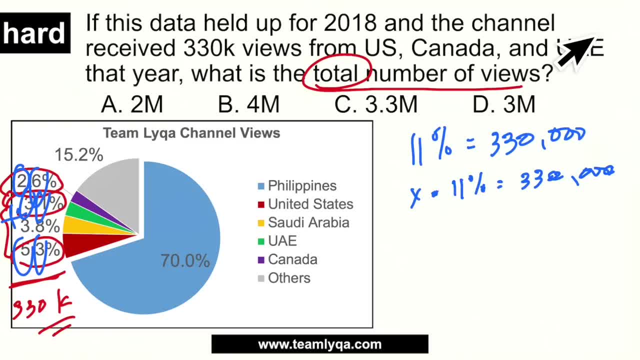 yung ratio rotation technique natin, pwede nyo siyang gamitin dito? Ano ibig sabihin? nun, Ganito lang, itatapat mo lang siya. Kung 11% yung 330,000, okay, ilan yung 100%, Okay. 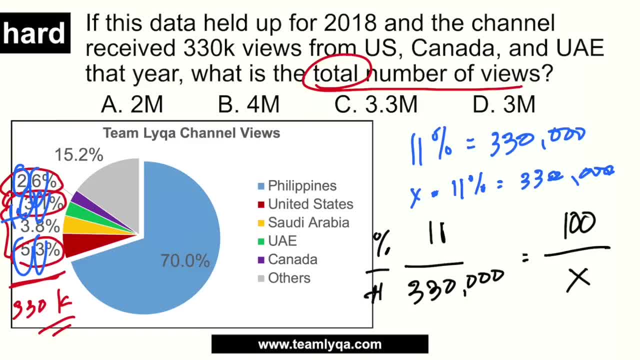 So again, eto yung percentage sa taas, eto yung number sa ilalim. Pwede mong gawing ganyan, Okay, Tinatapat ko lang siya Again. kung 11% is 330,000, ano ang 100%. Okay. 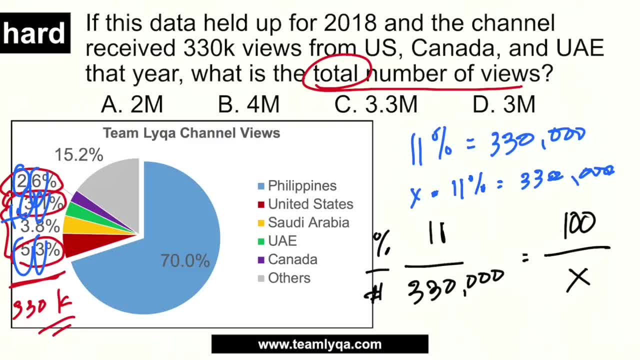 Tapos iiikot ko siya ngayon. Now, if you notice, madali naman kasi iiikot from here, kasi 33 tsaka 11, madali lang eh. 33 divided by 11 is 3, nadagdagan ko lang siya ng 4 na 0, so ganyan. 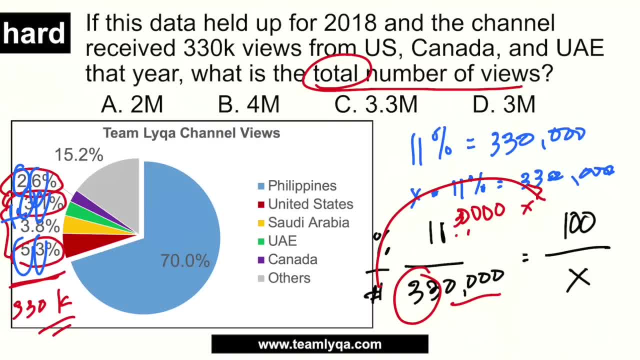 4 na 0,, so 30,000 times 100.. So yung 30,000, nadagdagan ko pa ulit ng dalawang 0. So magiging 3, 1,, 2,, 3, 4, another 2 zeros right there. 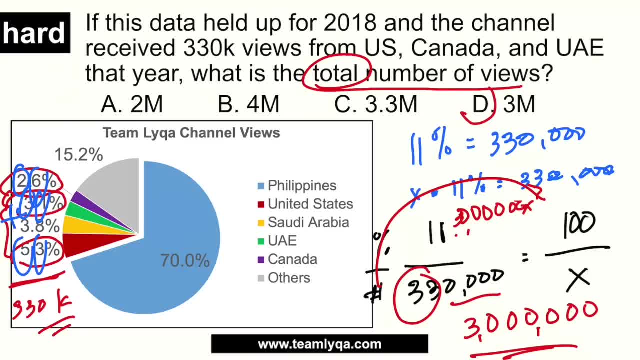 So my answer would be: 3 million views. letter D: Okay, So again ang ginamit ko ratio rotation. But again you can solve it like this, Para paraan lang yan. Maraming nagtatanong: sakit ko, paano ito i-solve. 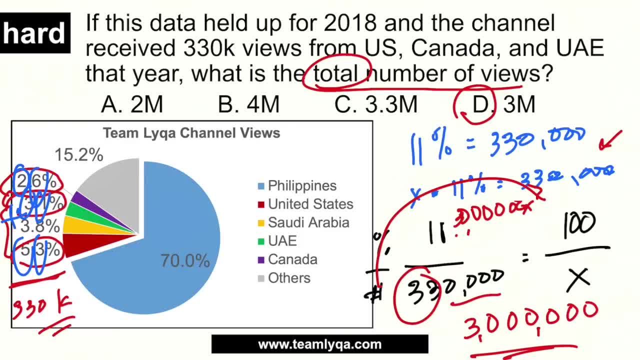 Ganito lang yung ginagawa ko sa exam. In most cases I guesstimate, Kasi kung mabilis ka mag-estimate, makukuha mo rin yung sagot, Kasi hindi pwedeng 2.. 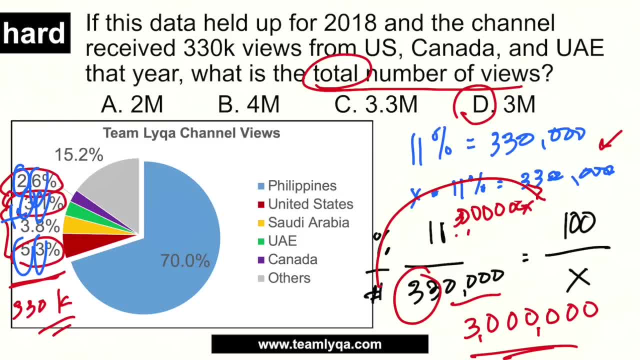 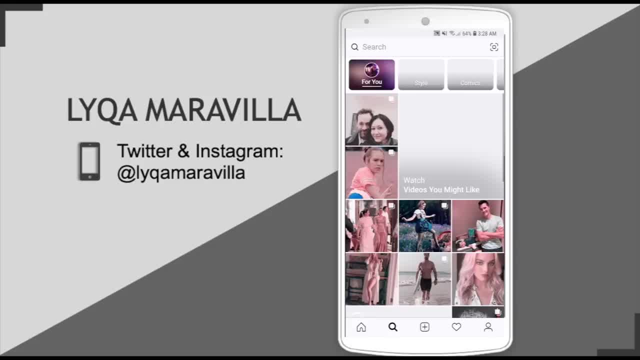 Masyadong mababa. Hindi pwedeng 4, masyadong mataas, So I would go for 3 million din. Now I hope nakuha nyo yan And if natapos ko yung aking free worksheet, ilalagay ko siya dito sa ilalim. 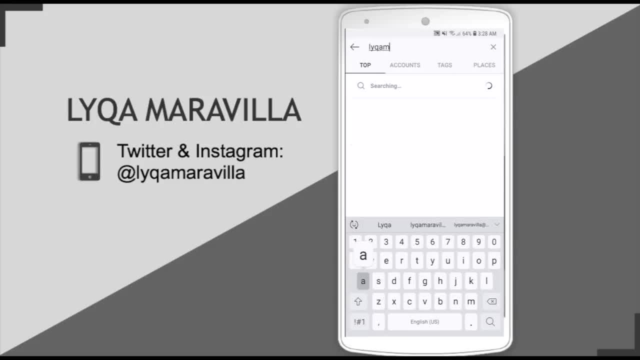 Nito sa description box ng YouTube video, And if hindi nyo yun makita or hindi pa siya ready, I will announce that din kapag ready na siya sa ating Facebook page, So follow me there na lang. I will also be posting more updates and more sample quizzes din on my Instagram account. 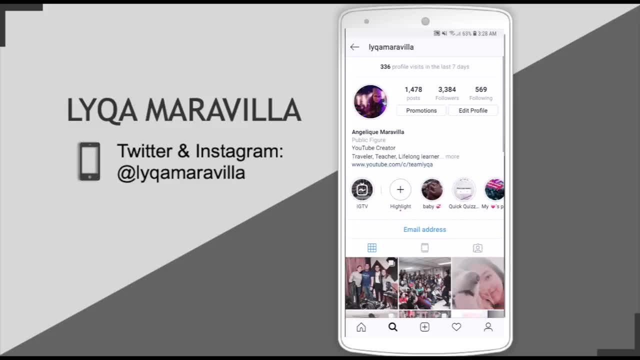 So if you don't follow me at, follow me at Laika Maravilla for the quick quiz function On Instagram. I hope to see you there. Magandang way yun for you to check kung natututo kayo. 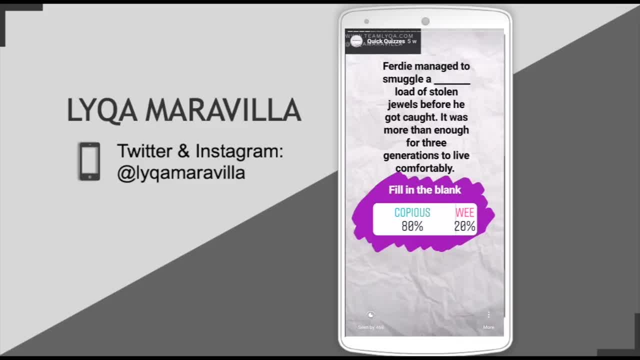 And for me din to gauge kung natututo rin kayo and which topics I should make videos of din sa susunod. Alright, I hope you learned something today. If you did, click thumbs up, Make sure that you share this video with your friends. 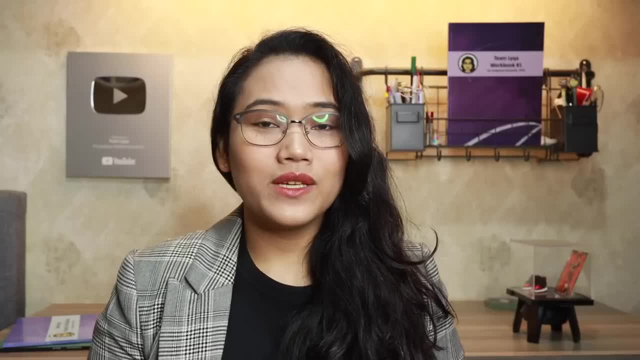 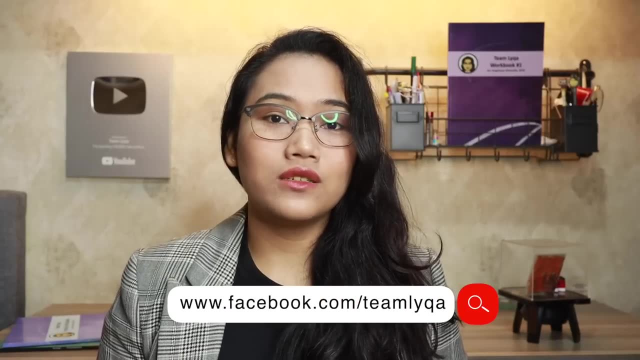 I don't know kung mag-e-examine sila. That way, mas maraming tayong matutulungan. And, as always, if you want to reach out to me directly, maybe find out how to get the reviewers that I made, or join the online or live review events, you can go to wwwfacebookcom.